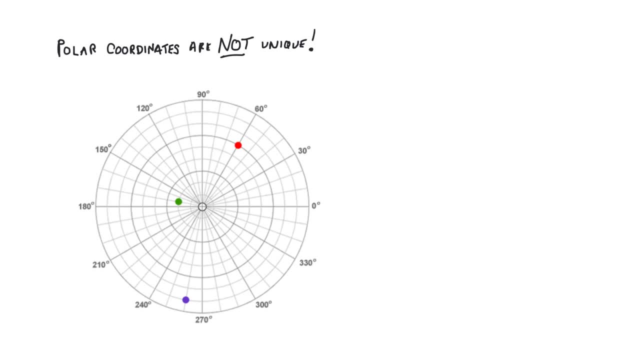 I wanted to make a quick video to explain how polar coordinates are not unique, So here's a polar graph with three different points. Let's first focus on coordinate A. The typical way to describe the coordinates at point A would be using its radius, which is six if you count out. 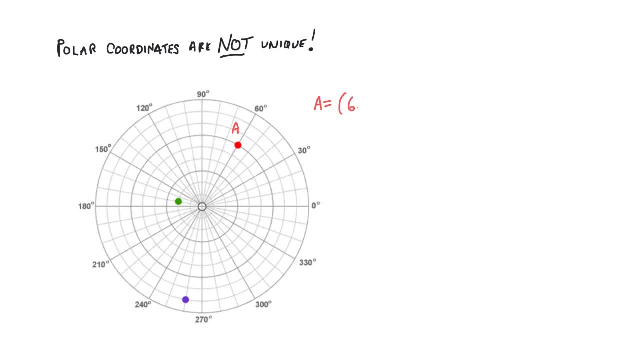 it's six circles away from the center, and then its angle, which is 60 degrees, measured counterclockwise from the positive x-axis. However, you can also be a little strange and instead describe it as 6,420 degrees, since an angle of 420 degrees would wrap all the way around. 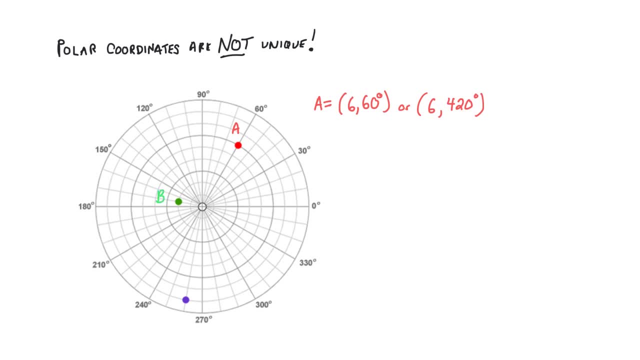 the x-axis 360 degrees, plus a little extra Meanwhile. point B: the typical way to describe that coordinate would be a radius of two and then an angle of 170 degrees, again measured counterclockwise. However, if you wanted to use a negative angle, you could come backwards 190 degrees and you'd 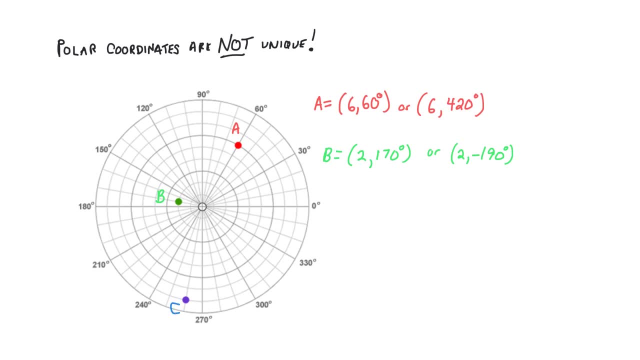 still end up at point B. It's the same. Meanwhile, if we look at C- in blue, because I can't find purple- C has a radius of eight, So the typical way to describe that coordinate would be eight comma and the angle is 260 degrees. However, 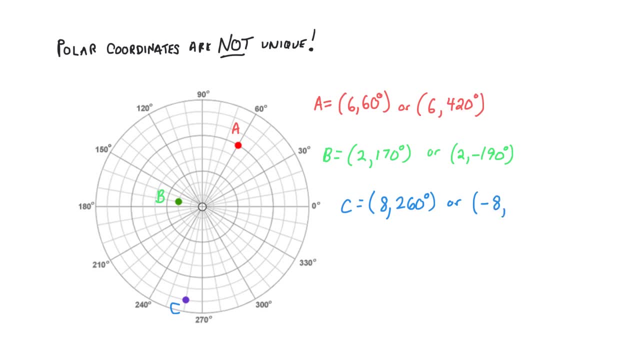 you could also describe it with a negative radius. So when we think about a negative radius, the way to think about it is a positive eight is on the positive x-axis, while a negative eight is actually moving out along the negative x-axis. So we're starting. 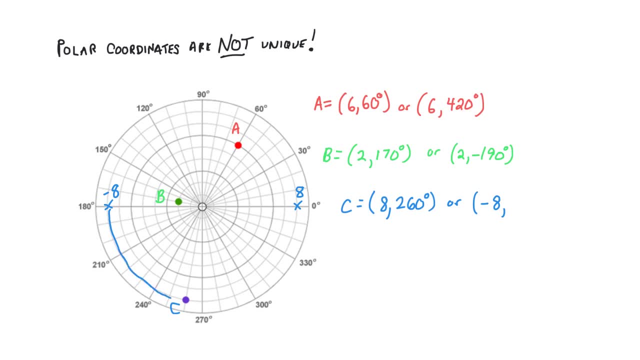 over here and then we're wrapping counterclockwise, assuming we want to use a positive angle to end up at point C And the distance that I would have to wrap along from negative eight all the way to point C is going to be negative eight, So we're going to wrap counterclockwise. 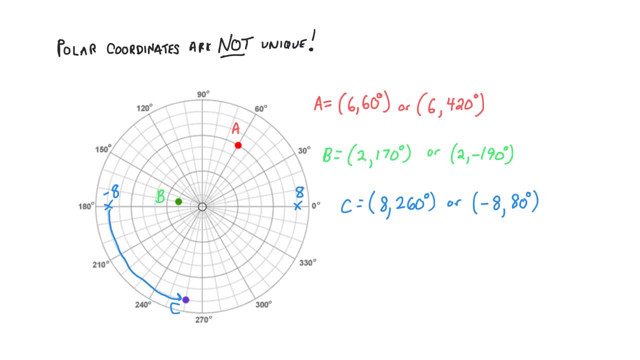 which would be two, the, Then we're going in towards the other side and then positive six. He's pointing up to a polar coordinate Cancer side with the Rusk to the left. I think this whole area at each point C is just going to be enough 80°. So that's yet another way. 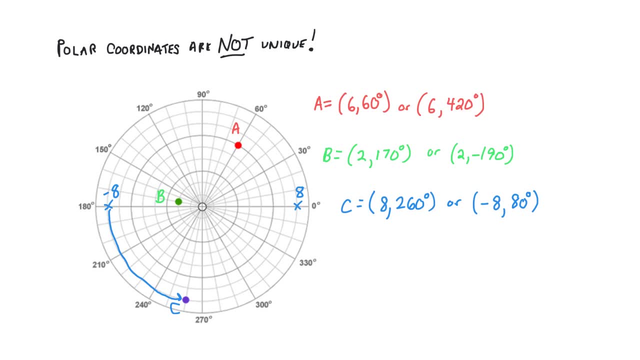 that I can describe the coordinates of point C. Now it's important to know that the first way that I described each one of these coordinates with a positive radius and a positive angle, with that angle being less than 360°, is the standard way to describe a polar coordinate.